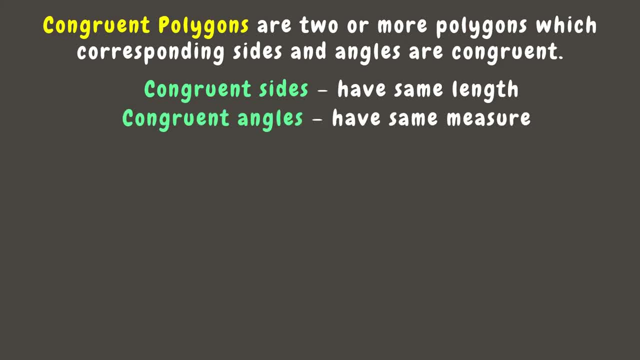 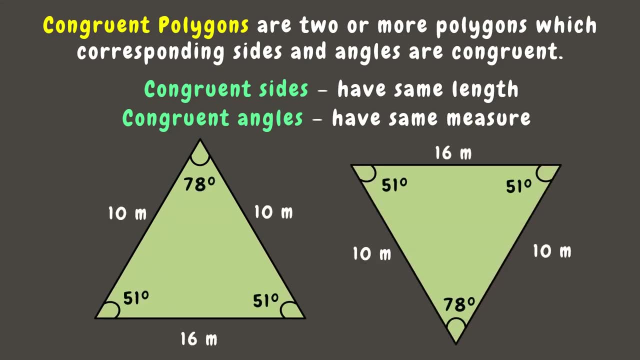 length, while angles are congruent if they have the same measure. For example, we have here two triangles. Let us observe. We can see that these two triangles have the same measurement of angles, where two angles are 51 degrees and one angle is 78 degrees. Therefore, 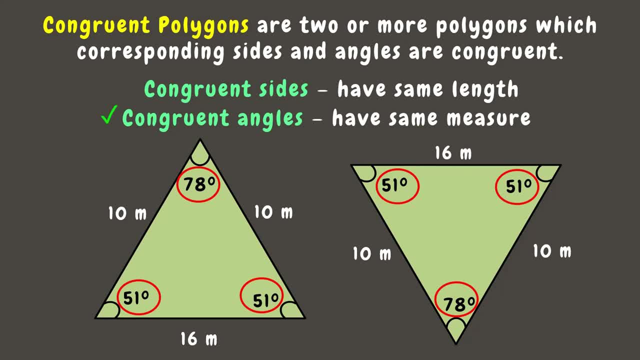 they have congruent angles. Also, we can say that their corresponding sides have the same length, where two sides are both 10 meters, while the other one is 16 meters. Therefore they have congruent sides. Since they have congruent sides and angles, it means they 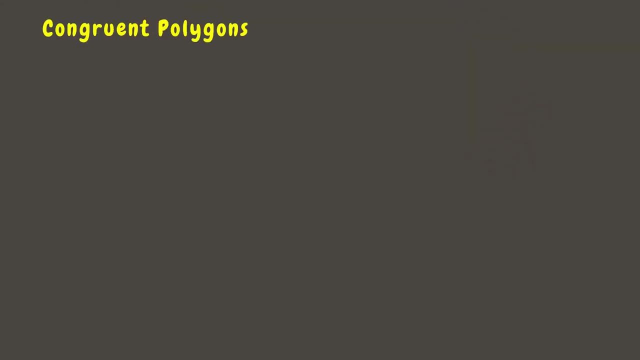 are congruent polygons. Now, congruent polygon necessarily must have the same shape and size. Going back to our sets of polygons earlier, we can see that the first set have the same shape. Also, the tick marks indicate that the corresponding sides of the two polygons are 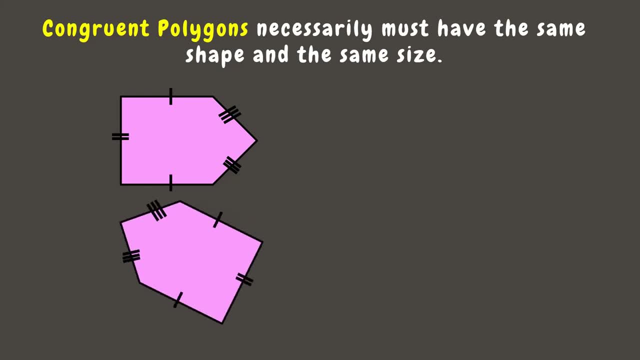 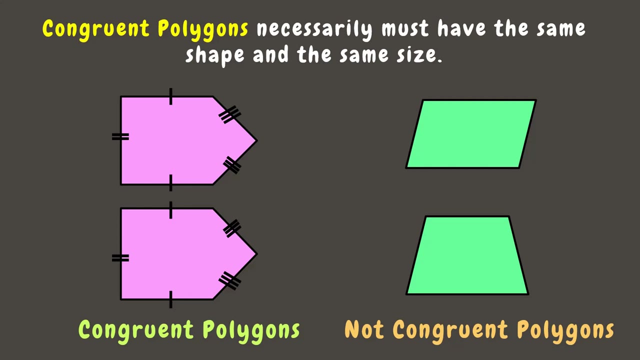 congruent and that the second polygon is just a rotated version of the first one. Therefore, they are congruent polygons, While the second set of polygons are not congruent since they don't have the same shape and size, which means they don't have congruent sides and angles. 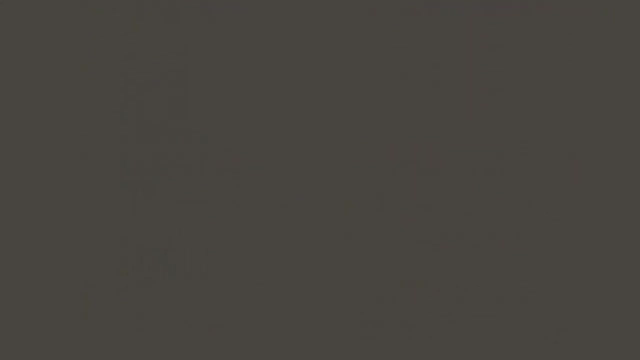 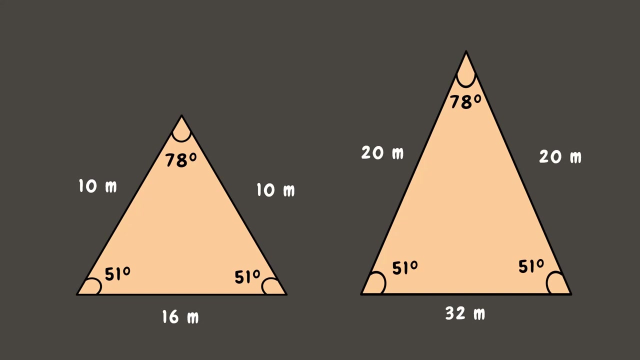 Let's have another example. Let's find out if this pair of triangles is congruent or not. First, let's take a look at their angles. Here we can see that they have the same measurement of angles. Therefore, they have congruent angles. Next let's take a look at their corresponding. 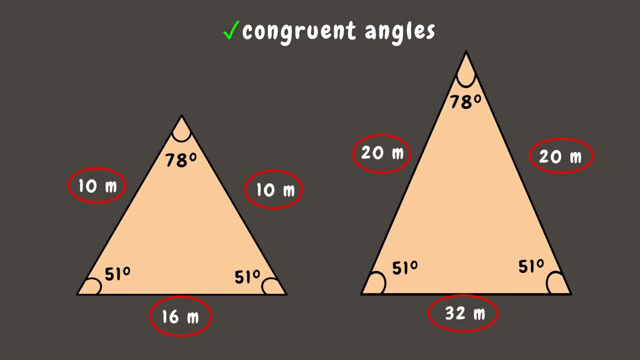 sides. Here we can see that their corresponding sides don't have the same length or measure, which means they are not congruent. Now, even though these triangles have congruent angles, we can still say that they are not congruent polygons, since their corresponding sides are not congruent.